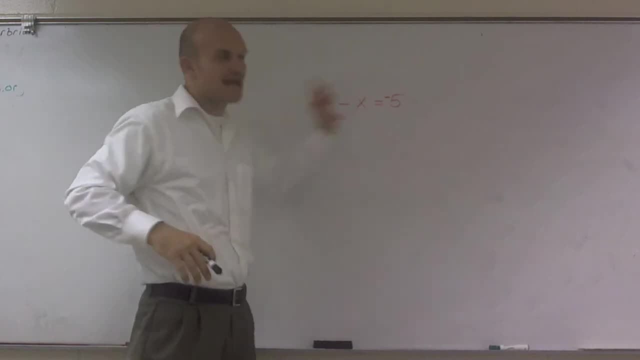 So what I would do is I would just get rid of, I would just multiply everything by 3, because if I multiply every term by 3, what now happens is these 3's cancel out. Right, Because 3 times x, divided by 1 times 3, the 3's will be 3 divided by 3, which would be 1.. So therefore, I'm left with x minus x times 3 is 3x equals a negative 15.. 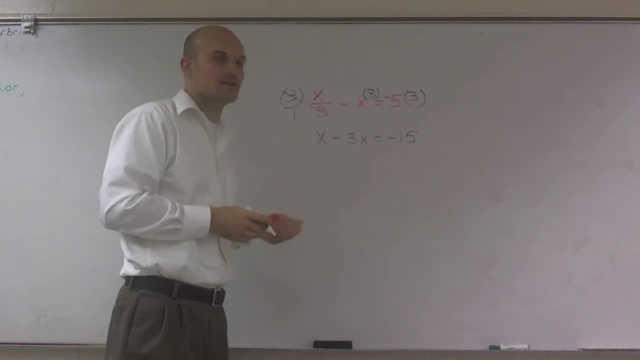 Now what I can say is x minus 3x is going to equal. if you have x and then you subtract 3x, you're left with a negative. 2x equals a negative 15. Then from here I can divide by negative 2.. 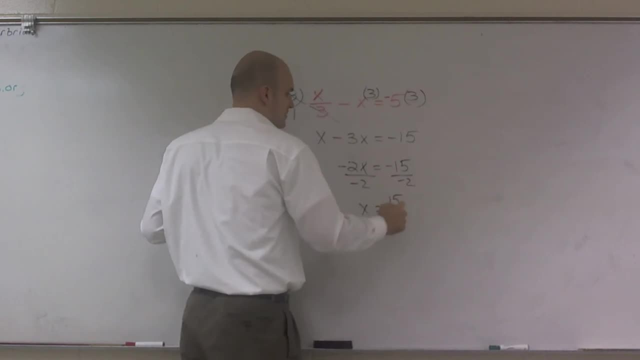 And I get: x equals a positive 15 halves, or you can write that as a decimal approximate or a decimal as 7.5.. So that's how you can solve that problem when you have two variables and one has a denominator. 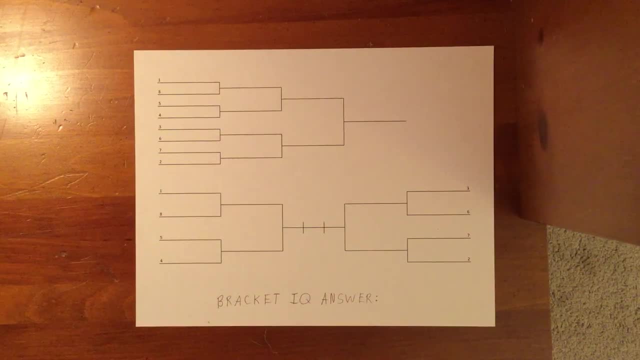 What's up guys? Welcome to Bracket Mania. Today we will be discussing the most common single elimination tournament. Today's Bracket IQ question is: what kind of tournament is the NCAA men's basketball tournament? Watch to the end to hear the answer. Let's get right to it. The single elimination bracket is the. 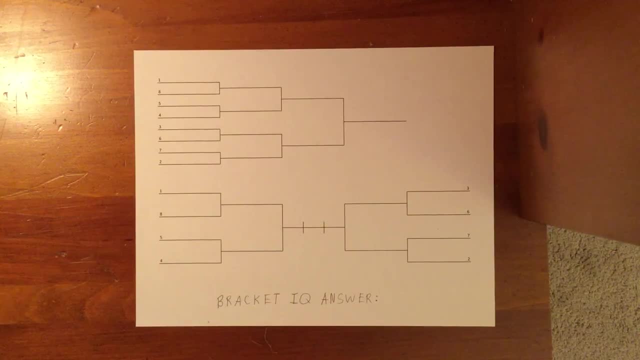 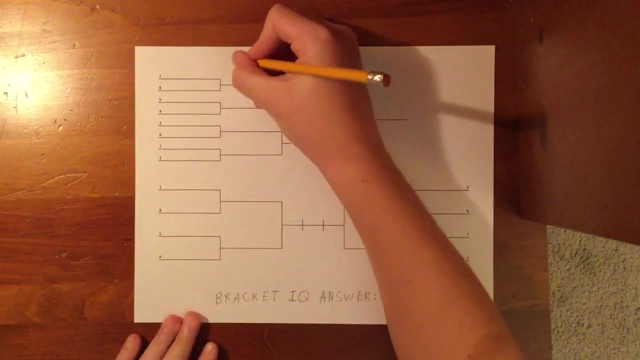 most commonly used tournament style as it's the least complicated. Many well-known tournaments use it, such as the NFL, college football and the knockout stage of the World Cup. On this page are two main formats of the single elimination bracket: The one side and the two side. 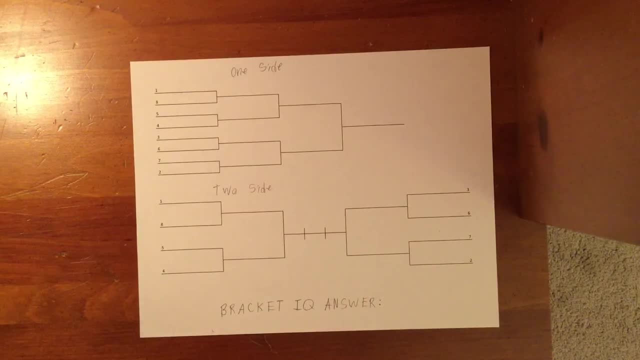 Each would work the same way. The person who wins in the match moves on to the next round. The person who wins the match moves on to the next round. The person who wins the match moves on to the next round. The person who wins the match moves on to the next round. 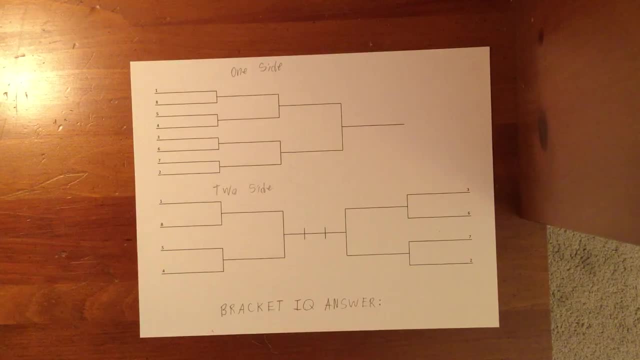 The next match, eliminating the loser until there is only one person left. The normal number of people in any tournament is by exponents of two. So two, four, eight, sixteen, thirty-two and so on would be tournament without buys. This one happens to be an eight-person tournament.